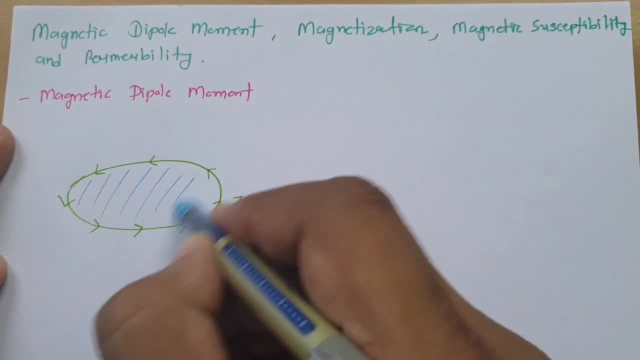 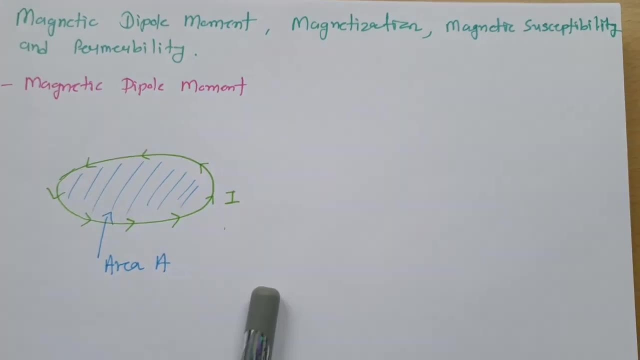 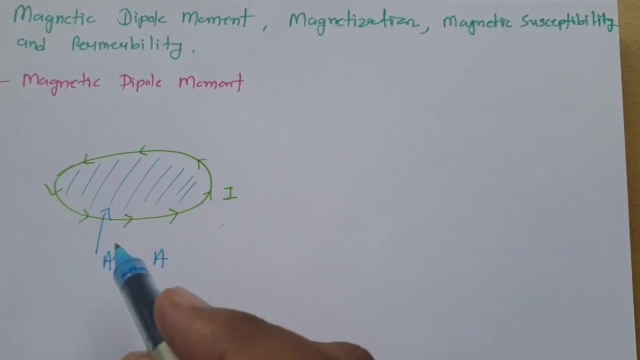 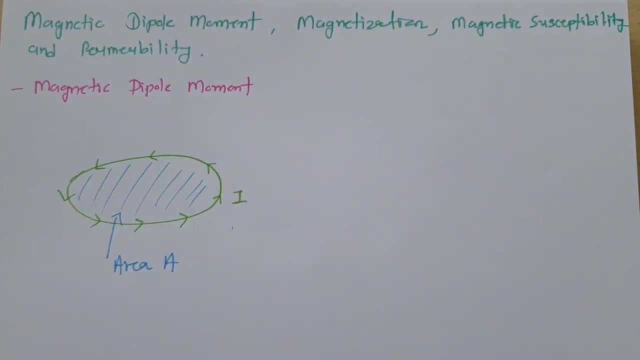 So I can say this cross-sectional area that is A And as per this cross-sectional area, A and current, I passing through this loop, magnetic dipole moment, magnetic dipole moment that will be current- into area. So magnetic dipole moment that will be current, I. 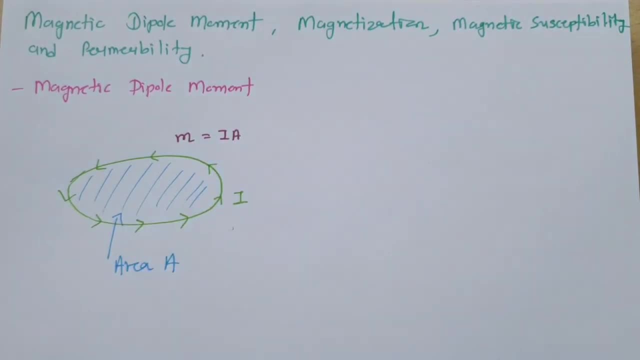 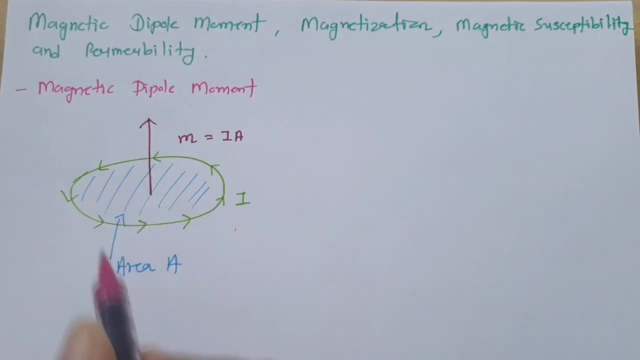 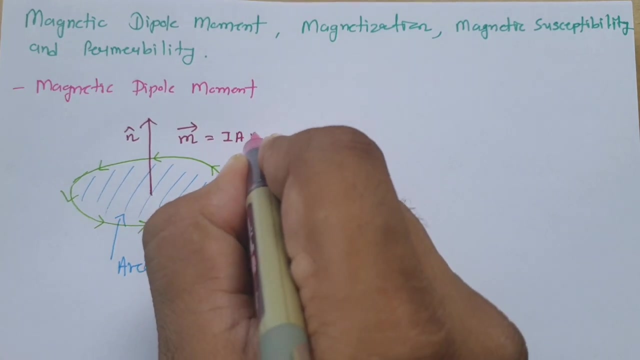 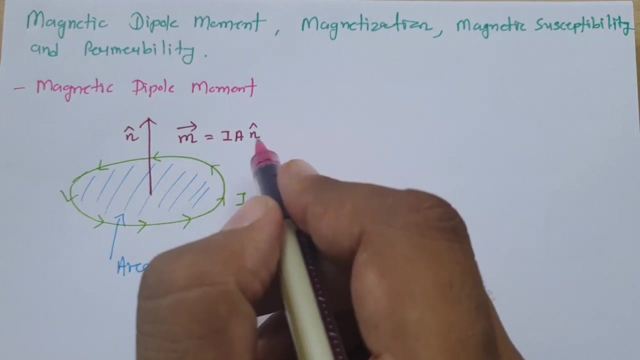 I into area A And if you want to calculate direction of magnetic dipole moment then direction of magnetic dipole moment that will be perpendicular to the surface. So if I say perpendicular to the surface is vector N, then magnetic dipole moment that is current into surface area of that loop and that will be there in the unit vector, direction of perpendicular to the surface. 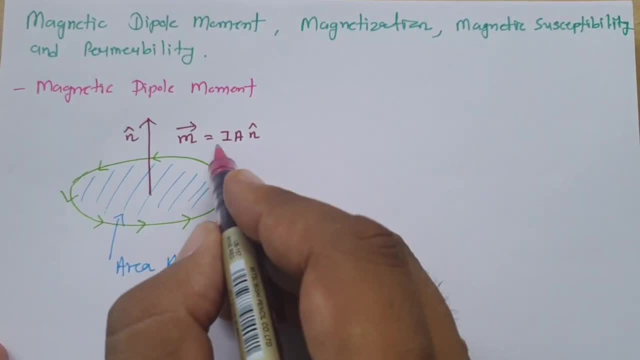 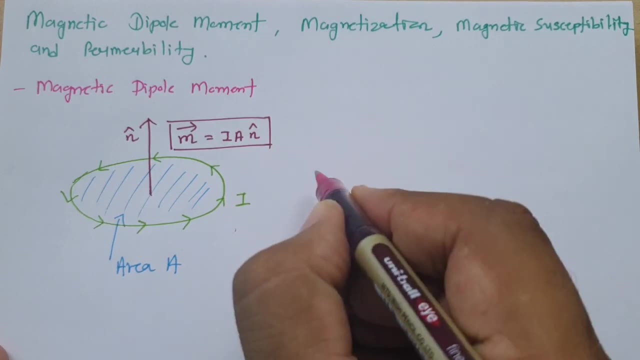 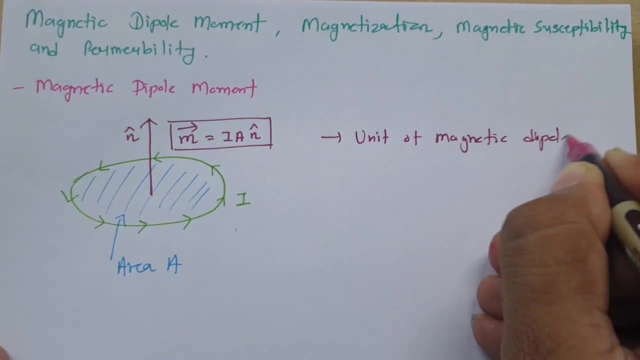 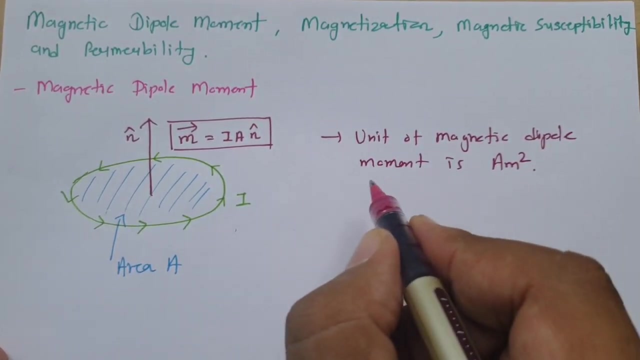 So this is what Magnetic dipole moment. it is current into area. So as per it is current into area, we can say its unit is ampere meter square. So unit Is ampere meter square and its direction is perpendicular to surface. 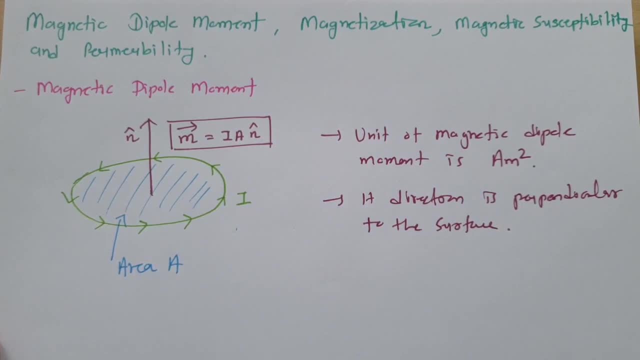 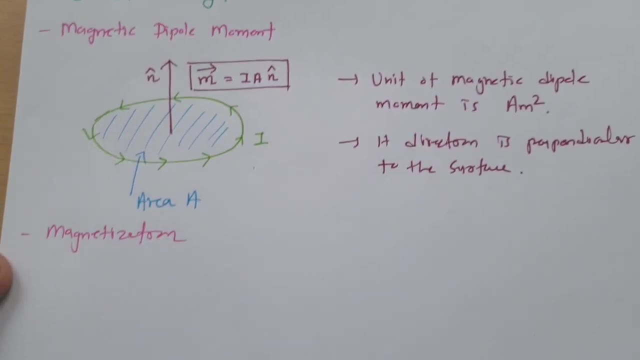 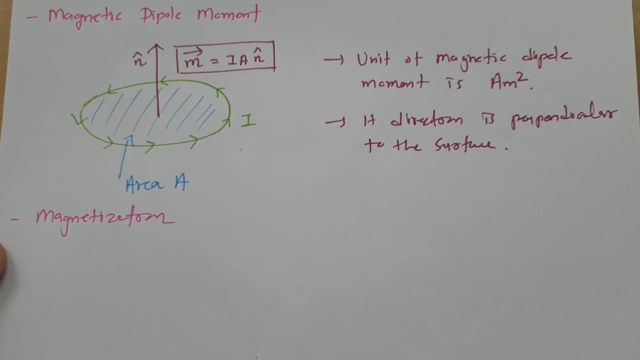 Now I'll explain you magnetization. So let me mention that first. Now see, magnetization That depends on material And usually if you have magnetic material then most of the magnetic field that is happening because of magnetization. So magnetization is purely depending on material. 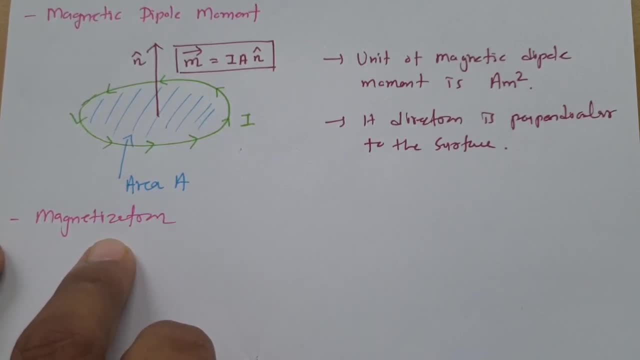 And for magnetic material Magnetization value that will be very high and that magnetization value will justify magnetic field, right? So you will be getting like how magnetization is very much important after a calculation which I'll be going to show you. 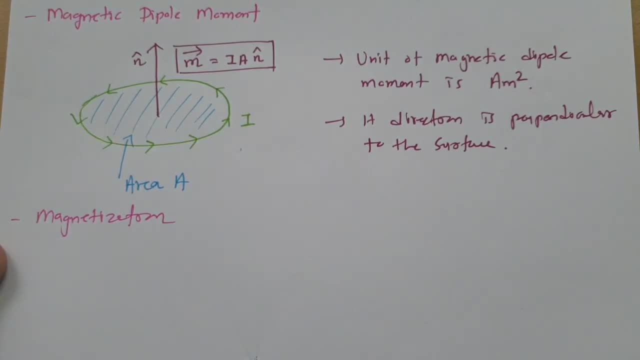 So, as I have told you, first point, that is, magnetization, is depending on material, So let me mention it. And then, last point is magnetic by the加油 Chromos, Monstrous Matrix, feminor animes is named magnetization. 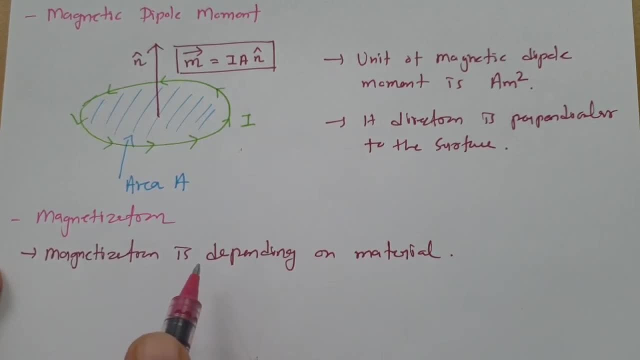 Now see what is magnetization. Magnetization is magnetic·dipole moment per unit volume. So basic definition of magnetization: that is magnetic·dipole moment per unit volume. So if you calculate unit of magnetization movement its unit is ampere meter square. so unit of magnetization that will be magnetic. 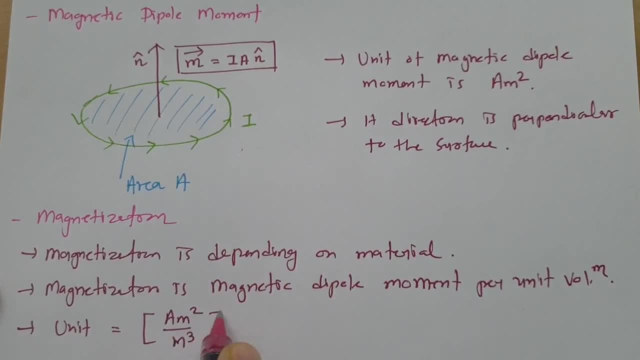 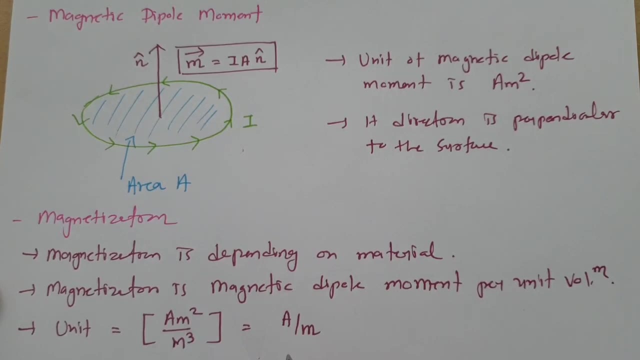 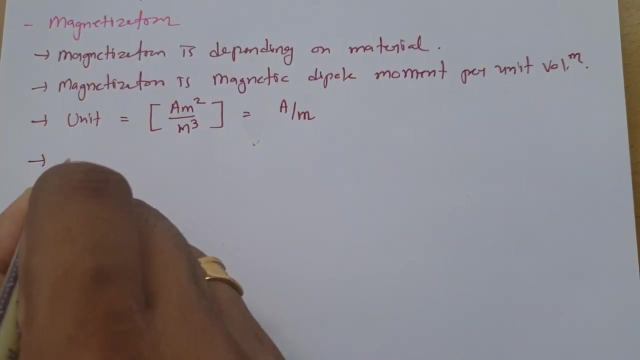 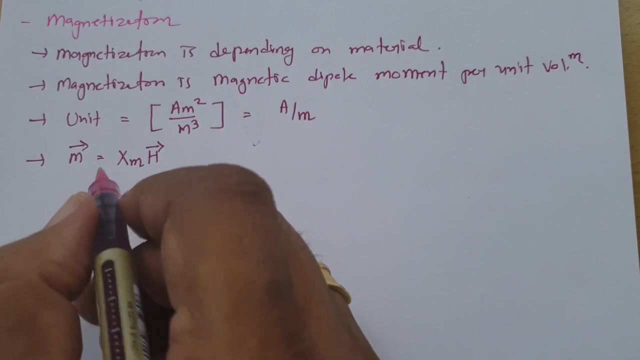 magnetic dipole movement divided by volume, so volume is having meter cube, so we can say unit of magnetization that is ampere per meter. right now, how to calculate magnetization? so for a calculation of magnetization we should know magnetic susceptibility of material. so magnetization, that is magnetic susceptibility into magnetic field, intensity, magnetization. 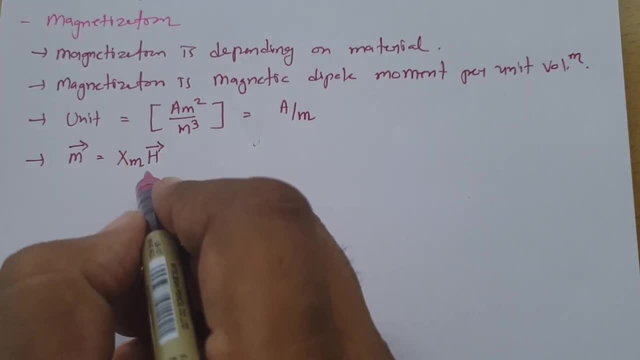 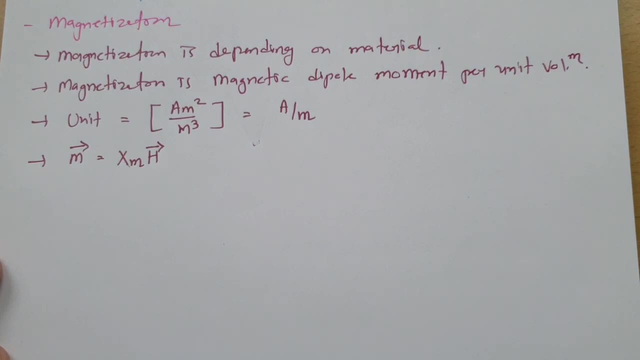 that is magnetic susceptibility, into magnetic intensity. so here this zeta m, that is magnetic susceptibility. so let me mention that so so, so. so now i'll try to establish a relationship in between magnetic susceptibility and permeability. so for that we need to calculate total magnetic field. so how much magnetic field will be there? 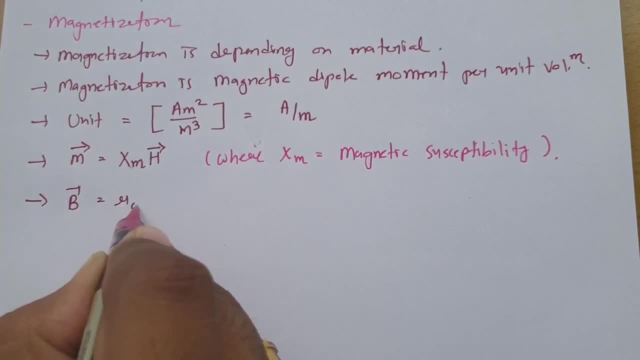 magnetic field that will be mu zero into h plus magnetization- see magnetic field- that will be mu z. usually we say that it is what mu 0, mu r h right, but practically it is mu 0 into h plus m, where m is magnetization right. so if you substitute this mu 0, h plus m is magnetic susceptibility- into h. 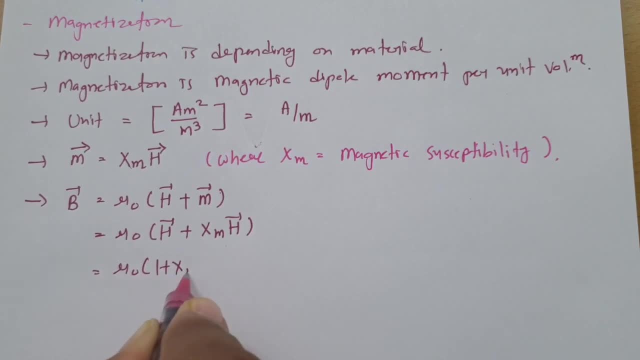 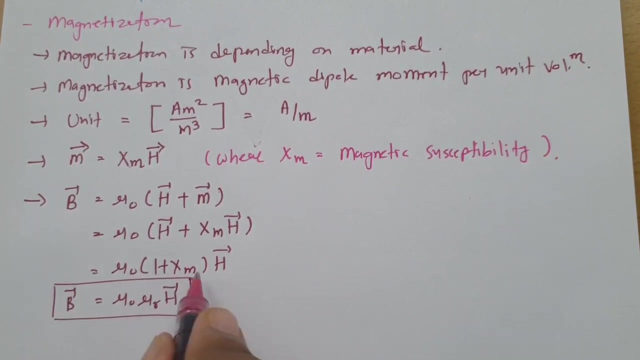 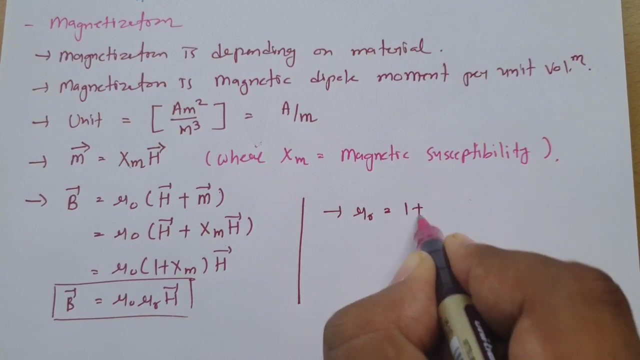 so we can say: this is mu 0 into 1 plus magnetic susceptibility into h, and this is what mu 0- mu r h. so magnetic field that is mu 0- mu r h, and where mu? r is what? 1 plus magnetic susceptibility. so mu r, that is 1 plus magnetic susceptibility, and mu? r is even referred as